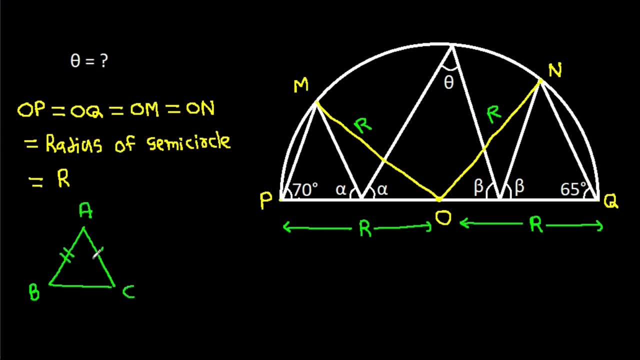 B, C. if AB is equal to AC, then these two angles they will be equal. so here in triangle it is OMP we have. OM is equal to OP, that is R, and this angle is 70 degree. so this: 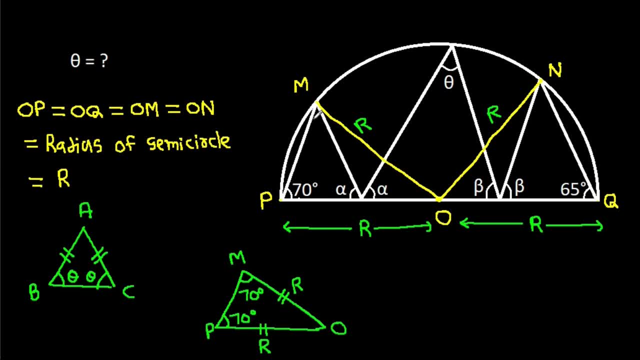 angle, it will be also 70 degree. this angle, it will be 70 degree here degree and inter angle, ONQ, it is ONQ, we have ON is equal to OQ, that is R, and this angle is 65 degree. so this angle, it will be also 65 degree. 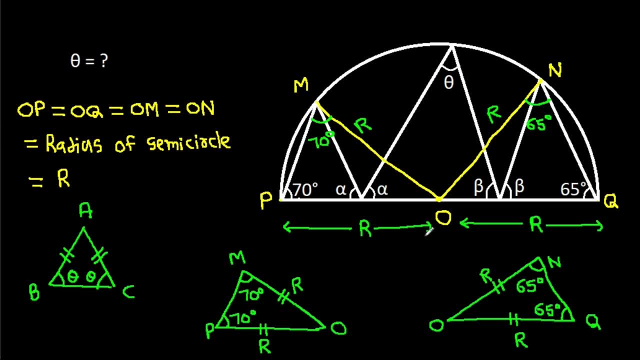 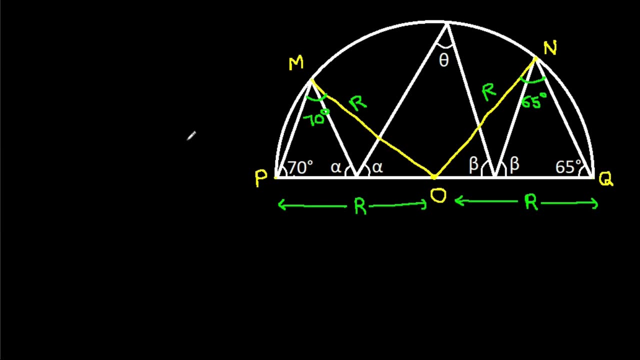 This angle, it will be 65 degree. and now inter angle OMP: it is OMP, that is R, and this angle will be 65 degree. Now inter angle OMP: it is OMP, that is R and this angle is 65 degree. so this angle is. 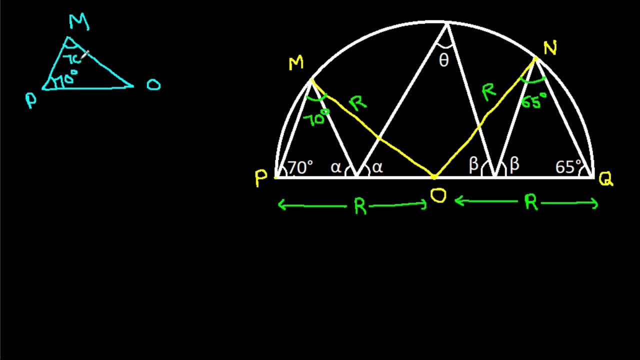 70 degree. this angle is 70 degree. so this angle, it will be 180 degree minus 70 degree minus 70 degree, that will be 40 degree. so this angle, it will be 40 degree and inter angle ONQ. 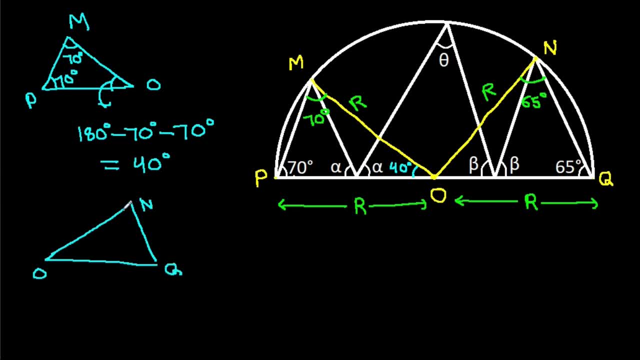 It is ONQ. this angle is 65 degree. this angle is 65 degree, so this angle, it will be 180 degree minus 65 degree. minus 65 degree, that will be equal to 50 degree. so this angle, it is 50 degree. 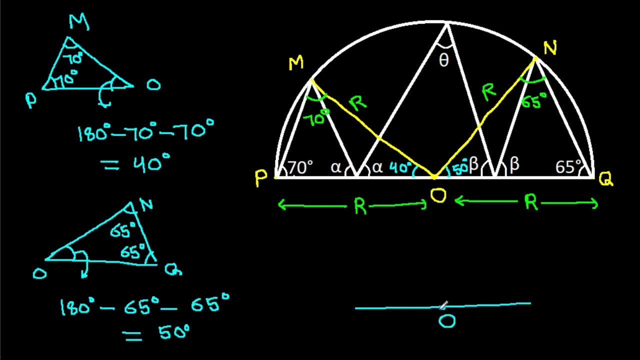 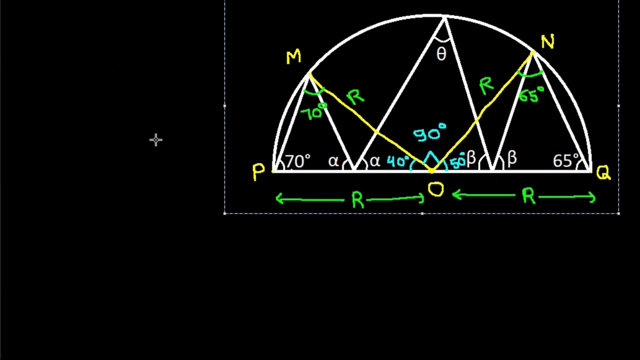 And now at point O, this angle is 40 degree, this angle is 50 degree, so this angle, it will be 180 degree minus 40 degree, minus 50 degree, that will be 90 degree. so this angle, it will be 80 degree minus 40 degree, that will be 90 degree. so this angle, it will be 90 degree. and 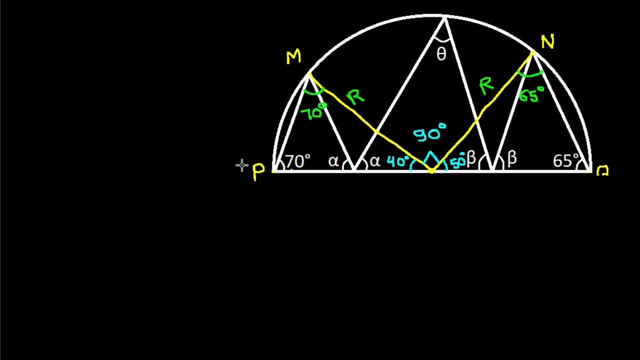 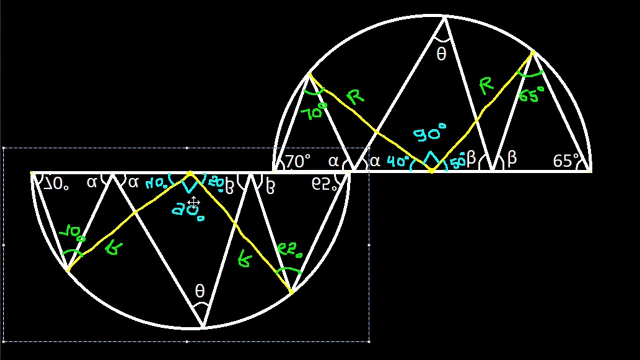 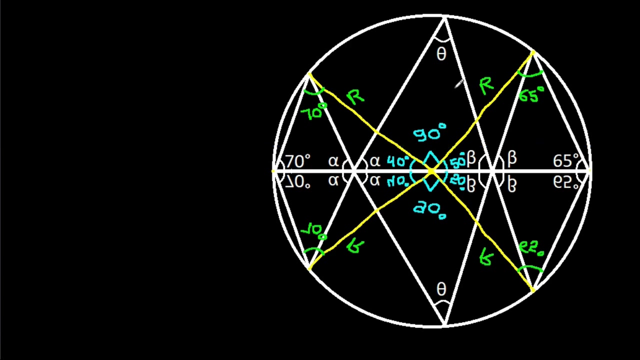 that will be 9 degree. So Они ARE THESE CIRCLES. ARE THESE CIRCLES NOW? NOW, IF WE- This is Suppose- this point is A, this point is B and this point is C and this point is P, this point is Q, then in PQ and AB, these two angles, they are equal. that is Antha, So AB it will be. 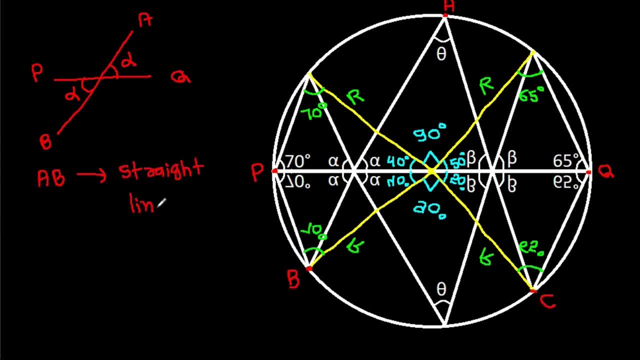 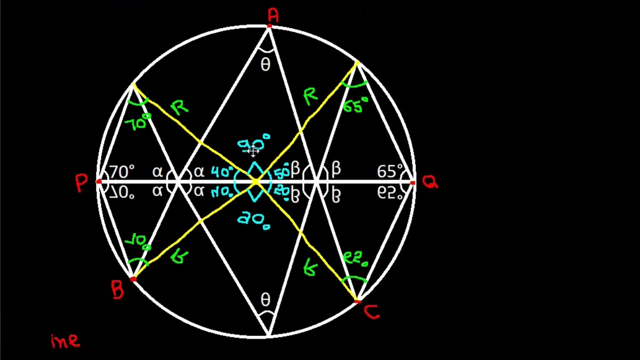 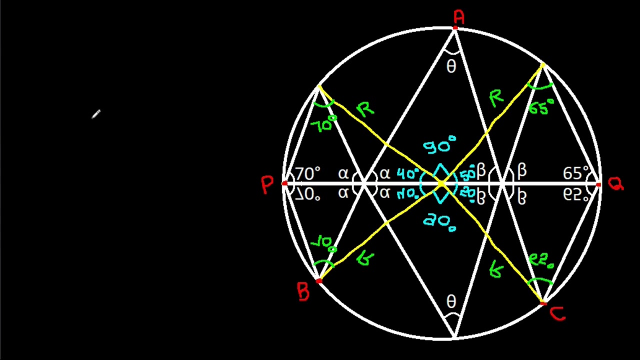 a straight line and also in PQ and AC, these two angles, they are equal and beta that means AC, it will be also a straight line. and now in any circle, if any chord AB is making an angle of theta on the circle, then it will.